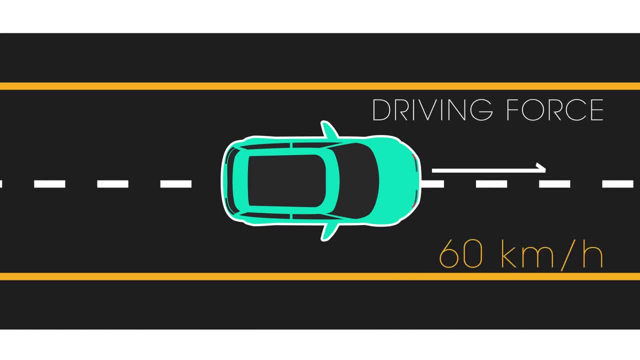 60 km per hour, The forward force from the engine is greater than, equal to or less than the backward frictional forces. If you said greater than, you may be confusing force and momentum. The moving car has a forward momentum defined by its mass times, its velocity, But 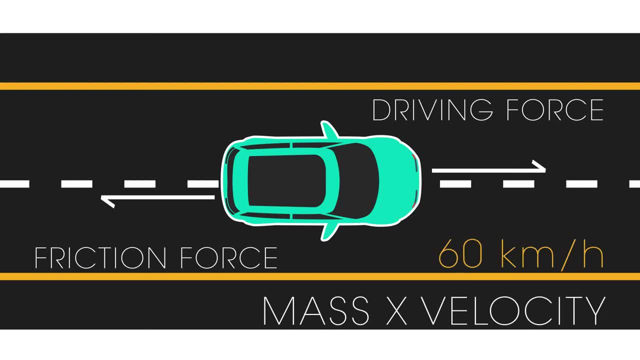 because it's not accelerating. its velocity is a constant 60 km per hour. The car is moving at a constant 60 km per hour. The forces must be balanced, so there is no net force on the car. If the engine force were higher, the car would be getting faster, increasing its speed and 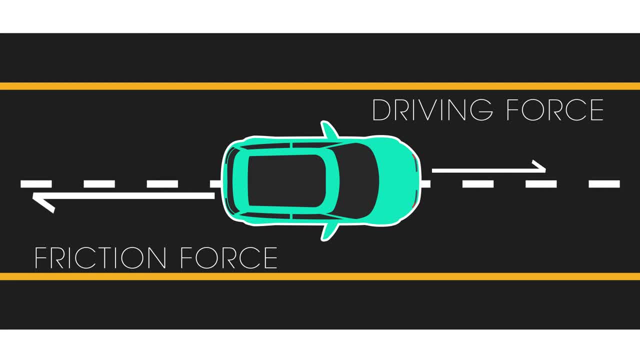 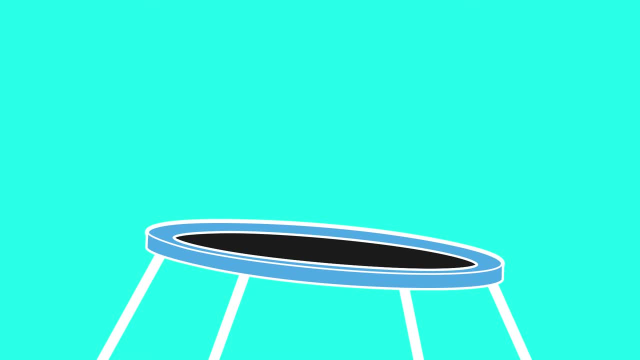 momentum, And if lower, the car would experience a backward force and be slowing down. If you like, momentum is a measure of how difficult it is to stop a moving object. The more massive the force is, the more it will be able to move. If you like, momentum is a measure. 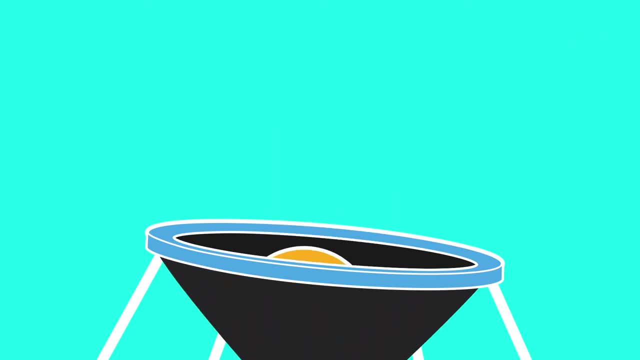 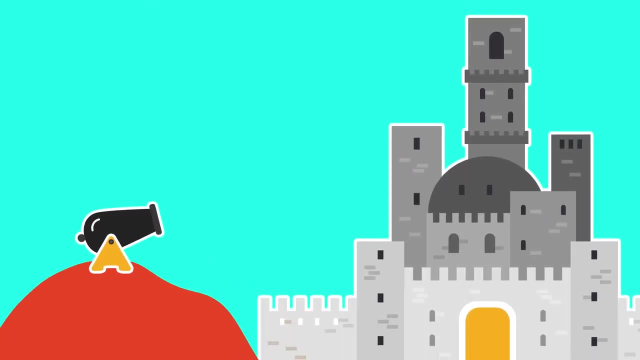 of how difficult it is to stop a moving object. The more massive the force is, the more it will be able to move. The more massive it is and the faster it is moving, the harder it is to stop it. Think of firing a cannonball at a castle wall, If it were made of wood or travelling slowly. 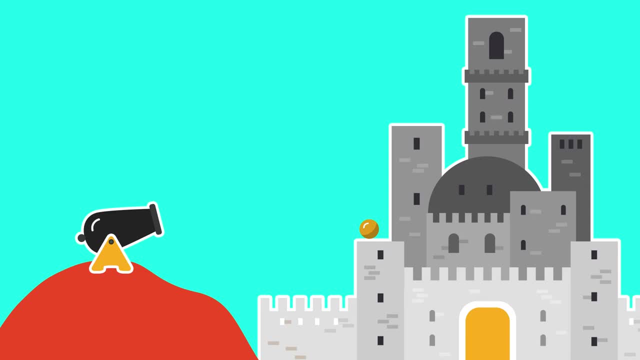 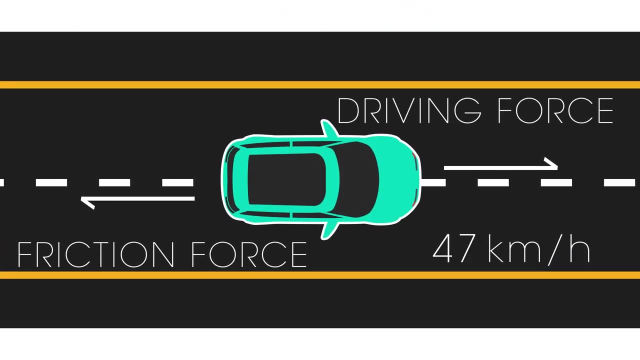 the wall can easily stop it, But if it's made of a dense metal and travelling fast, it could go right through the wall. So try this one. The car is slowing down. The arrow shows its velocity, which is getting lower. The car is moving at a constant 60 km per hour. 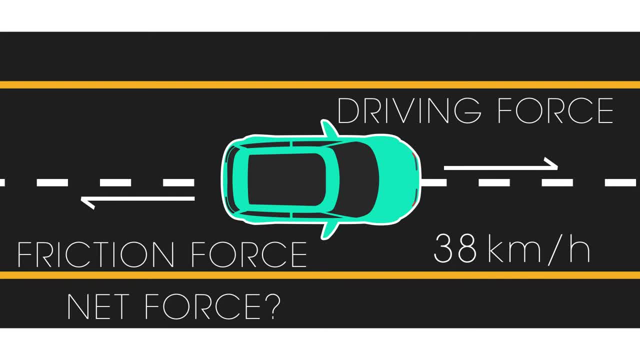 What direction is the net force on the car? Is it forwards or backwards? Yes, the force has to be against the forward motion to enable the car to slow down. And what about the momentum of the slowing down car? Yes, because the car is still moving forward. 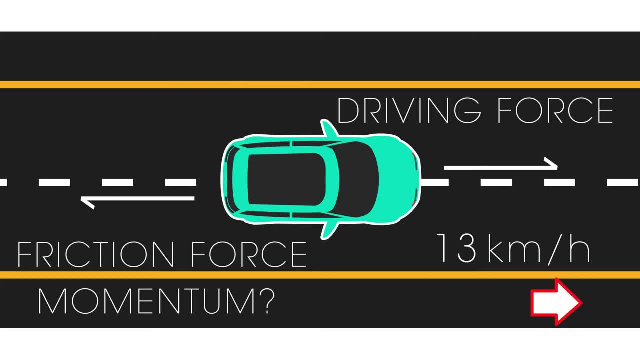 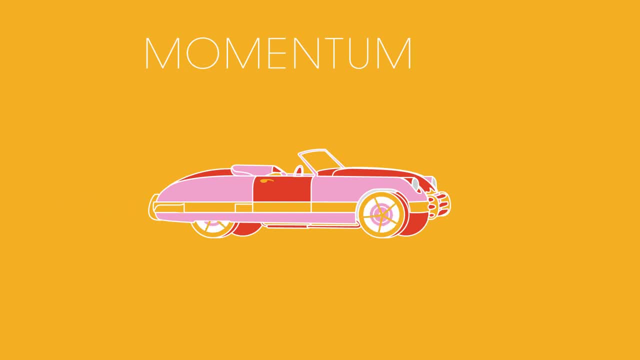 even though it's slowing down, it still has a forward momentum. All moving objects have the momentum in the direction of movement. A stationary object has a momentum of zero. We calculate momentum using this equation: Momentum p equals mass m times velocity v. This can also be displayed in a formula triangle. 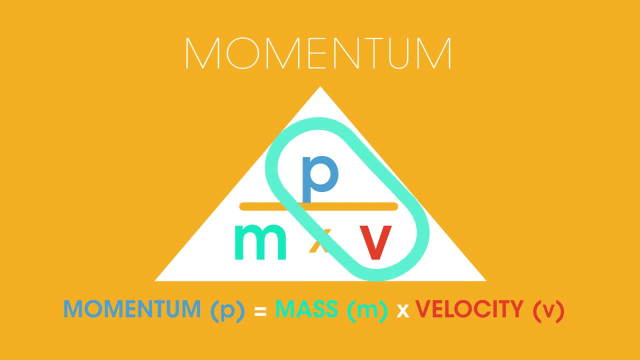 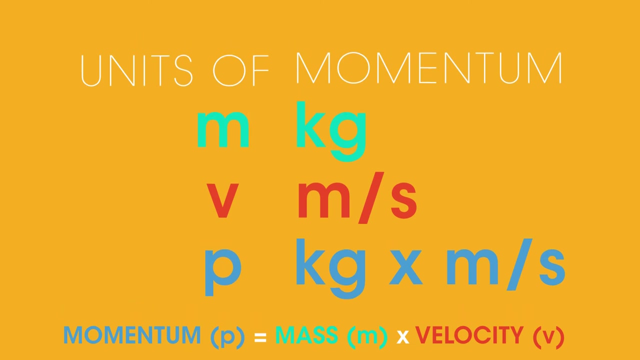 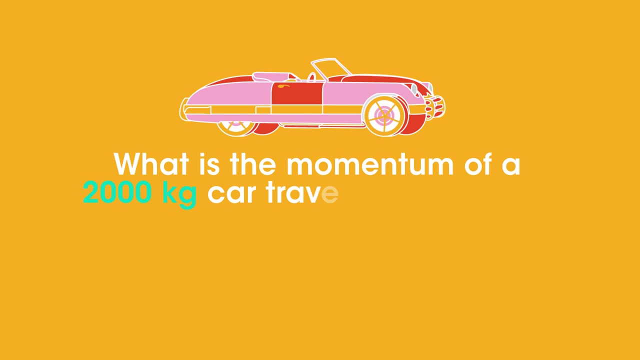 like this. So mass equals momentum over velocity and velocity equals momentum over mass. So what are the units of momentum? Mass is measured in kilograms and velocity in meters per second. So momentum equals kilograms times meters per second. Now try this example: What's the momentum of a 2000 kilogram car travelling at 7 meters? 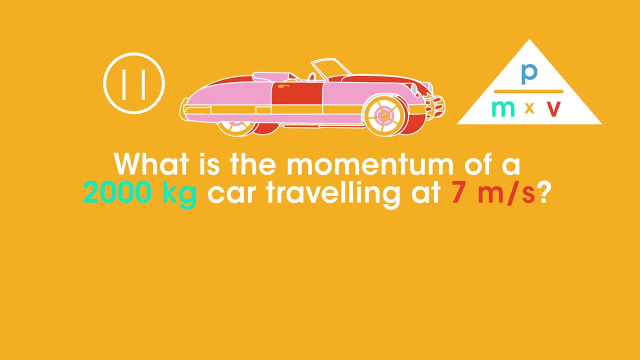 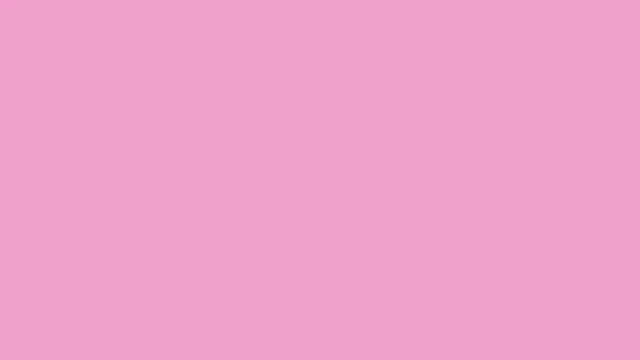 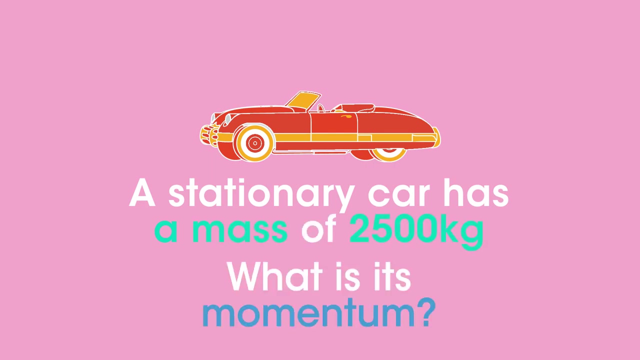 per second. Pause the video while you work it out. How about this one? A stationary car has a mass of 2,500 kilograms. What is its momentum? Pause the video and work it out. The car is not moving, so its velocity is zero and so it has no momentum. 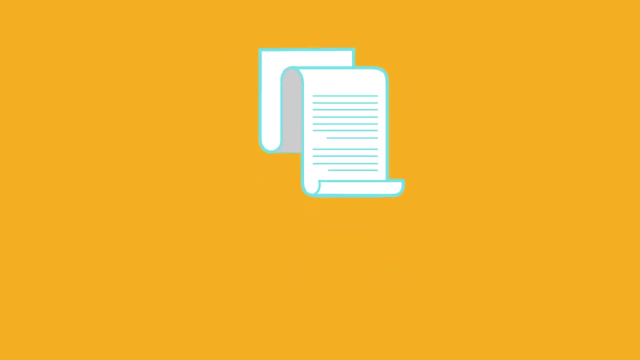 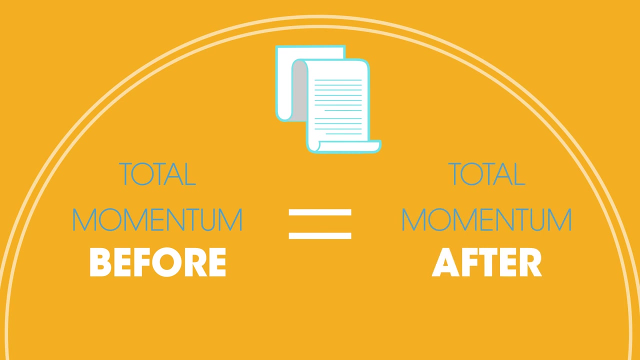 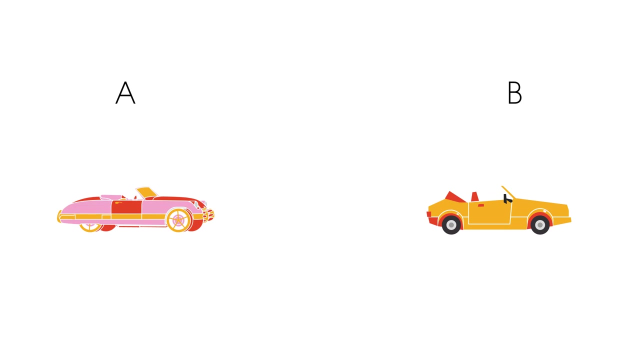 So what's the law of the conservation of momentum? In a closed system, the total momentum before an event is equal to the total momentum after an event. Let's look at how to apply this. Two cars of equal mass- 800 kilograms- collide Before the collision. car B is at rest while 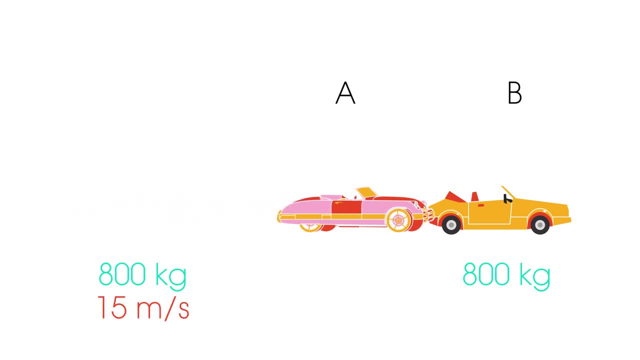 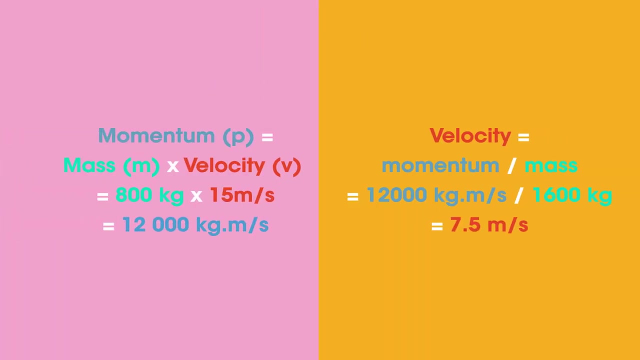 car A is travelling at 15 meters per second. Calculate the momentum of car A. What is the momentum of car A After the collision? the two cars are stuck together. Calculate the velocity of the cars after the collision. Pause the video while you work it out. 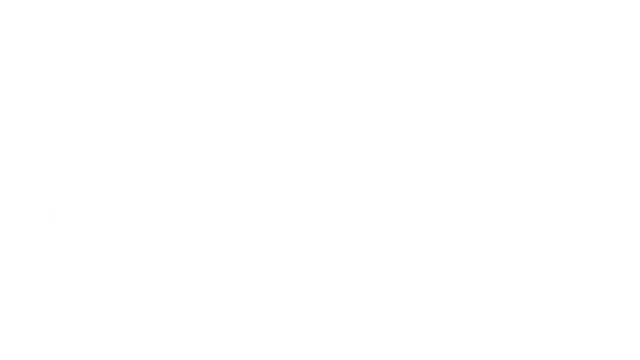 How did you do? Let's try another. Two toy passenger cars moving towards each other collide and stick together. Use this information to calculate the momentum of car A. What is the momentum of car A? What is the momentum of car B? What is the momentum of the cars after the collision? 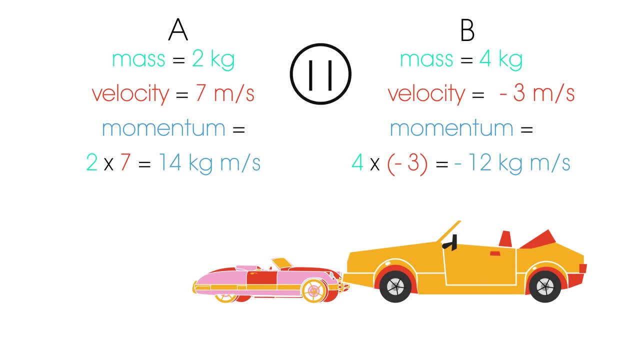 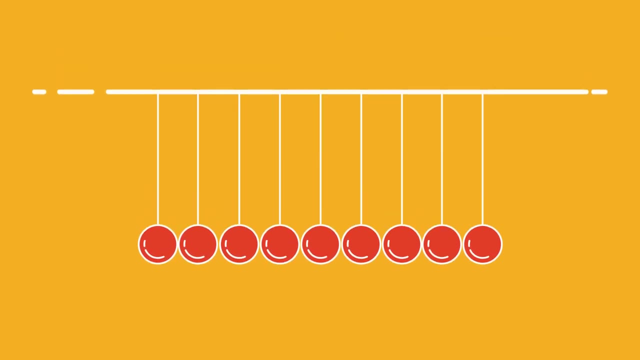 Pause the video while you work it out, Because car B is moving in the opposite direction to car A. its velocity is negative. Let's finish with this toy. Can you explain why the end ball moves off at the same speed as the colliding one?